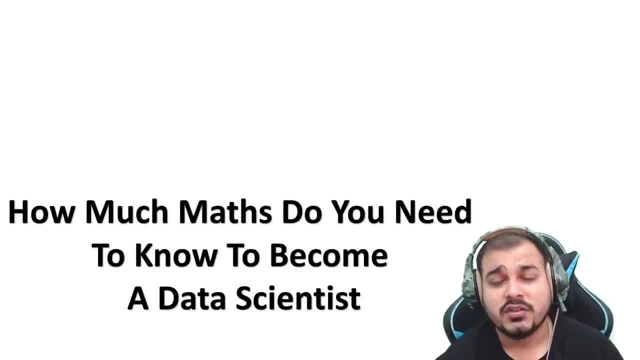 I did not had a good hold of maths, So can I cope with this when I'm actually trying to become a data scientist? Let me tell you guys, when I was actually in my school days- or college days like 10 plus 2, or engineering days- I knew maths. I used to practice a lot, but I never understood the 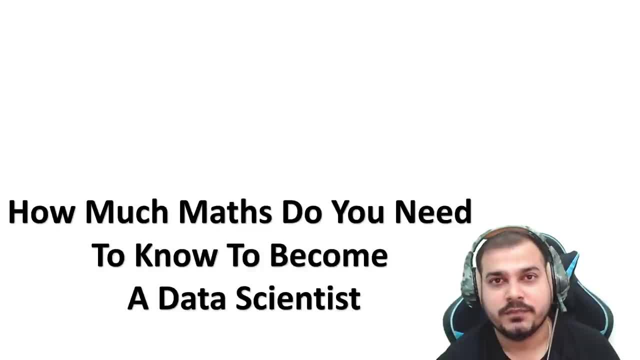 practical application of it. I never knew why differentiation was used. Probably I was not able to relate with a real world scenario. I was not able to relate with a practical implementation. That is the most common mistake that we usually do and many people does. You know when you are. 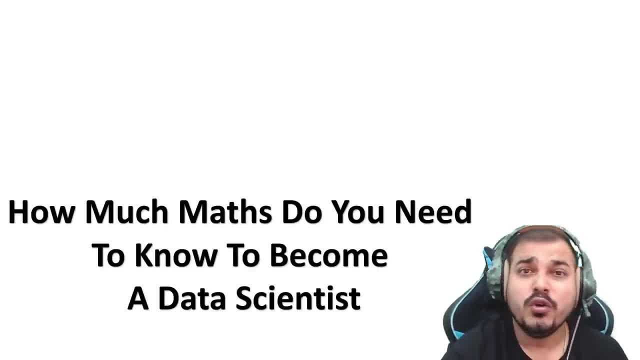 actually learning maths from your school days or college days. why you do not? why many people have been able to understand. they're not able to relate to it, And that is the reason why many people are afraid of maths. That's it, You know. but as soon as I learned data science, I was able to relate, so 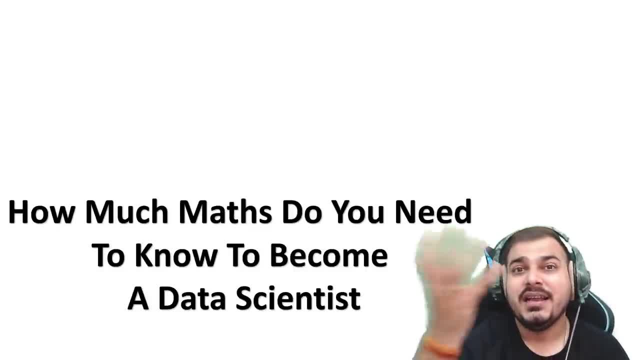 many topics because I had something I was using that in a practical real world scenario Stats. you know, I was able to apply the equation. I was now able to understand why differential equations are used, why integration is basically used for a specific purpose. And that was all possible when. 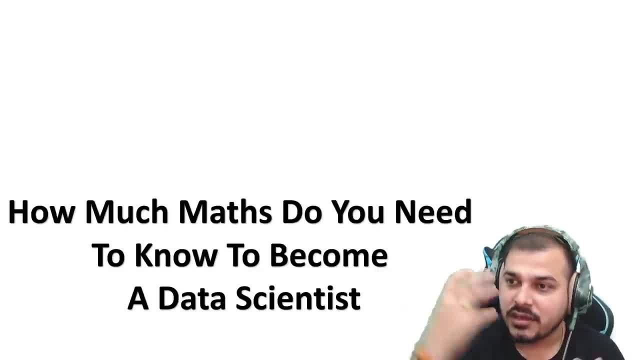 I started learning data science Because when I was learning a topic, I was able to relate it with a real world application. So in this particular video I'm going to cover how much maths do you require, or do you need, to become a data scientist? And remember, guys, this question was asked by 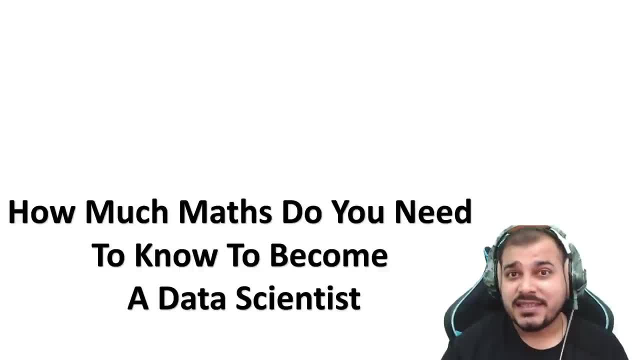 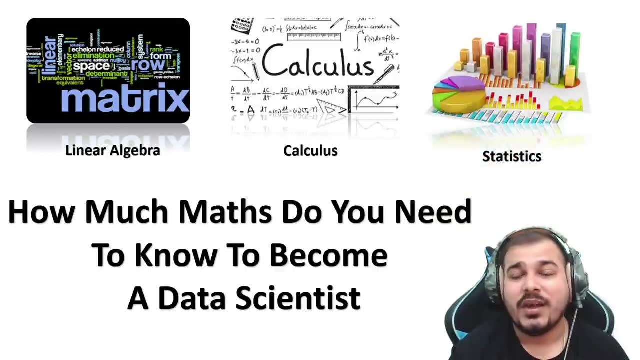 many, many people. What if I say: okay, the main thing in maths that you really need to know is basically these three things. One is: you know, and trust me, this is very, very much simple. One is linear algebra, One is calculus, One is statistics. 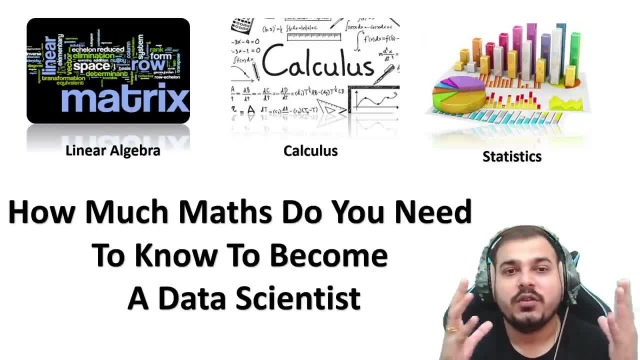 These are the main three sections. with respect to the maths that you're going to learn as a data scientist, Yes, your school knowledge, your college knowledge, will be definitely applicable, And there are many syllabus, many topics. that probably is basically getting covered, if you're 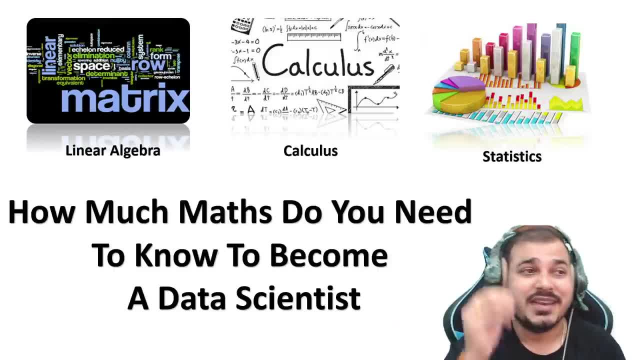 learning with respect to data science, But the main three subsection is linear algebra, calculus and statistics. And always remember, guys, do not learn this subject separately, Always try to learn it by learning. Suppose I'll give you an example. okay, Suppose I'm learning how does a neural network work In neural network, if I want, 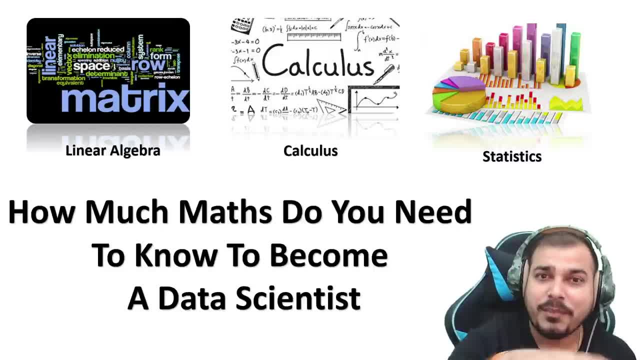 to understand how does gradient descent work, that part calculus will come. If I want to understand how the weights are getting updated, that part through back propagation calculus will come. If I want to see that how the inputs and the weights are getting multiplied, that part linear algebra. 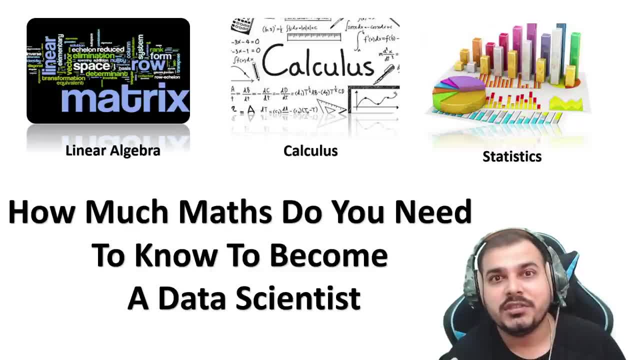 may come. You know, Suppose I'm solving a machine learning problem statement, I really need to visualize some kind of data. I want to analyze some kind of data. I want to do some kind of test like Z test, T test. That time statistics will come. Okay, Always understand when you're. 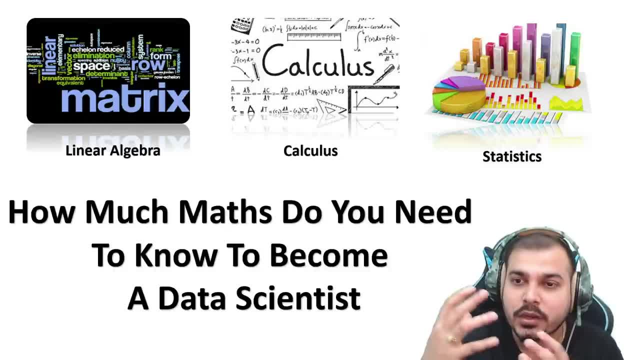 trying to learn in this particular manner, you'll definitely be able to relate it, because that time- suppose, if I'm learning differential equations when I'm learning how a back propagation will happen- that time I'll get a clear idea that how does partial differentiation and 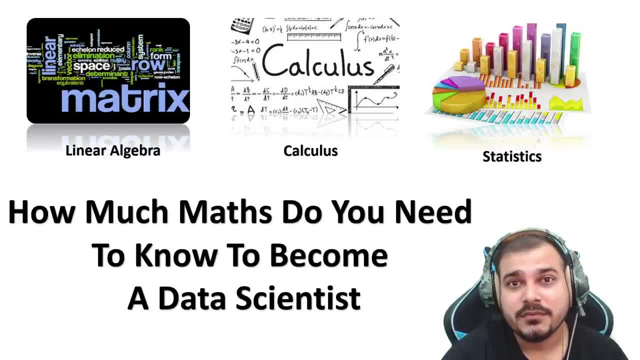 actually work and how it is related to a real world scenario. So never learn it separately, because these subjects are quite huge: How it is getting applied, how it is getting used in data science. that is the main thing that you really need to understand. Otherwise, if you do PhD also, 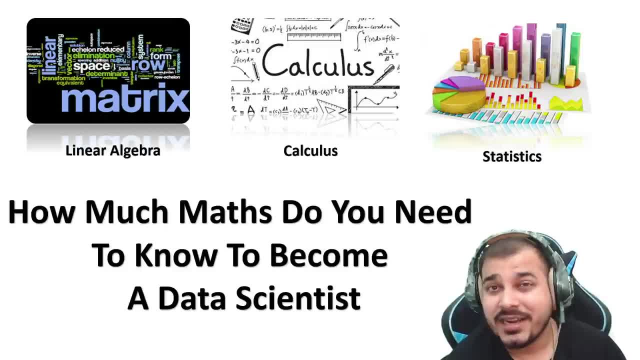 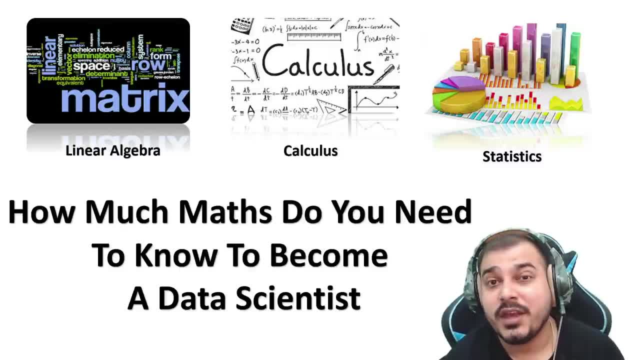 learn all the other things, that is, linear algebra, calculation of statistics, wherever it is required. Most of the time when you're learning machine learning, like if I take you an example of, there's an amazing algorithm in machine learning which is called as principle-competent. 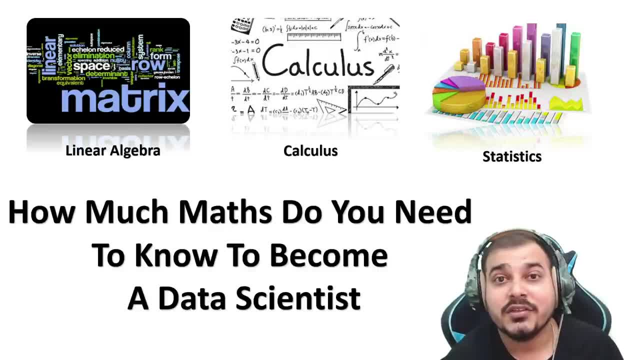 analysis And in principle-competent analysis you really need to understand about vectors. At that time I'll definitely try to use linear algebra At that time only I'll try to understand it. And when I'm trying to learn linear algebra at that point of time, definitely it'll be. 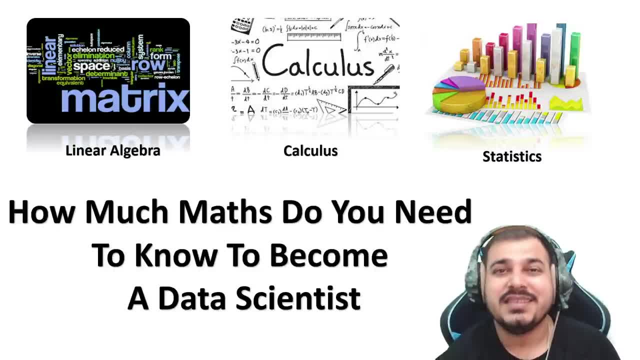 very, very helpful for us and we will be able to relate it. This is how I have actually learned. you know, I'll tell you how you should basically go ahead with what all resources you should basically refer, But let me give you one very good example. 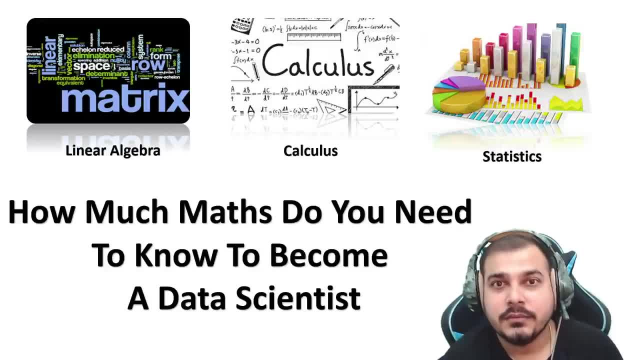 Okay, If you remember, guys, there is an algorithm which is called as linear regression, which is the most basic first algorithm In linear regression. you will be having calculus. you will be having linear algebra topics. you will also be having statistics topic. Now, how did I learn linear? 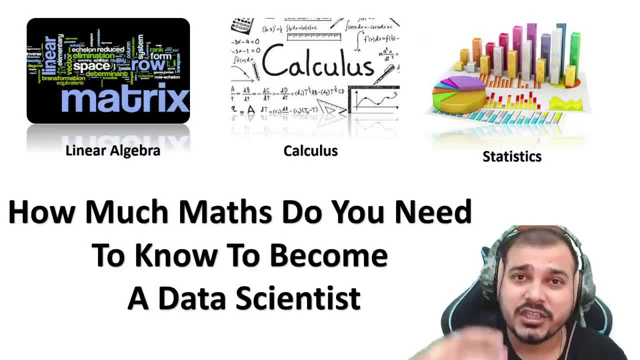 algebra, sorry, linear regression, Just understand. in linear regression you have something called as cost function. There the weight updation is basically happening by using this partial derivative which is involved in calculus. Now, I understood that particular topic when I was. 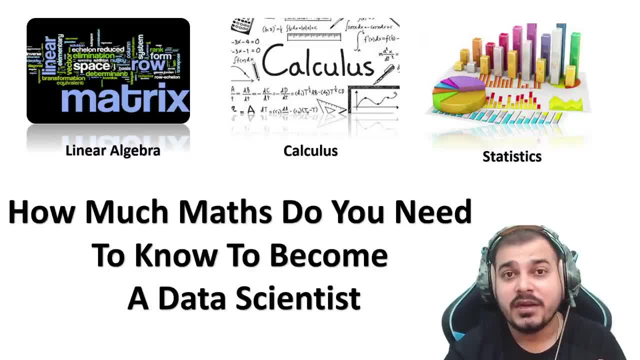 learning that particular algorithm. Linear algebra also, I'll be able to understand, because there we'll do a lot of different, different kind of weights, multiplication or coefficient multiplication. y is equal to mx plus c. Stats: how does the statistics different? different concept. 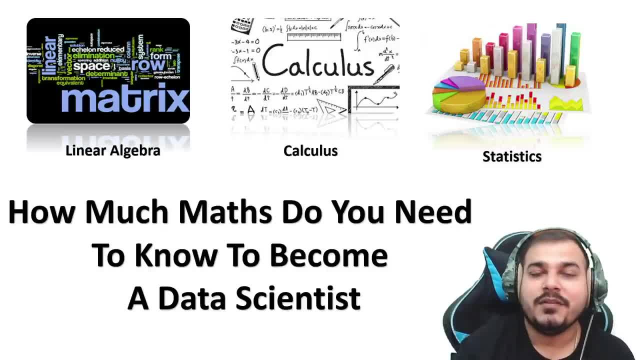 do we require Scaling in linear algebra? So that part- some of the statistics formulas- will definitely come because we are dealing with data right. So this is how, whenever I was learning one algorithm, I did not learn separately what is linear algebra separately In linear algebra also. 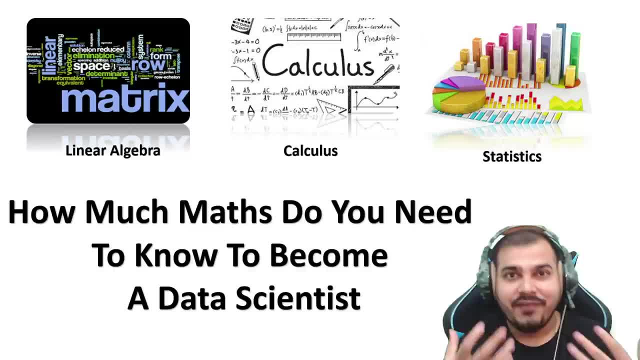 you have something called as vectors. Okay, Yes, I have learned vectors in my school days, but I was not ever able to relate it. So that is the reason why I'm saying you that never learn separately. Instead, learn it while you're learning, something like a machine learning. 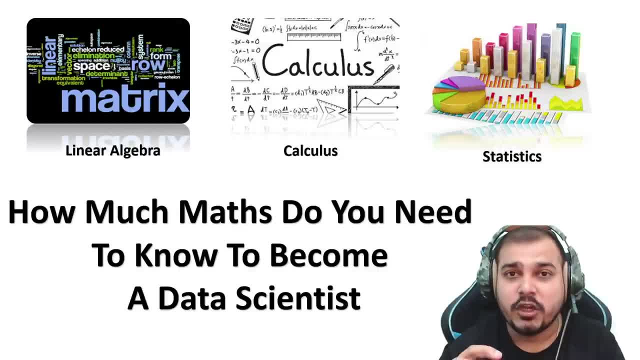 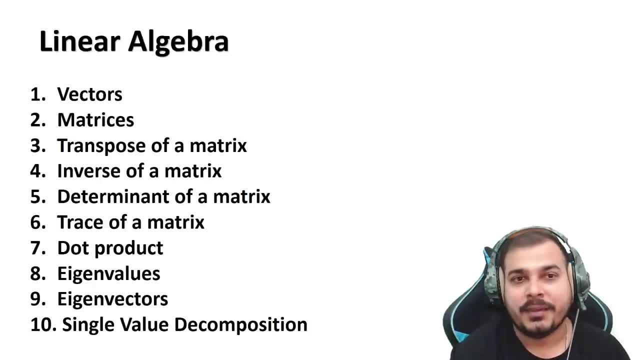 algorithm. I say that as reverse engineering. I pick up the main topic and then try to divide that into multiple pieces and try to learn each and everything. right Now let's go to the next step In linear algebra: what all things you really need to be good at? 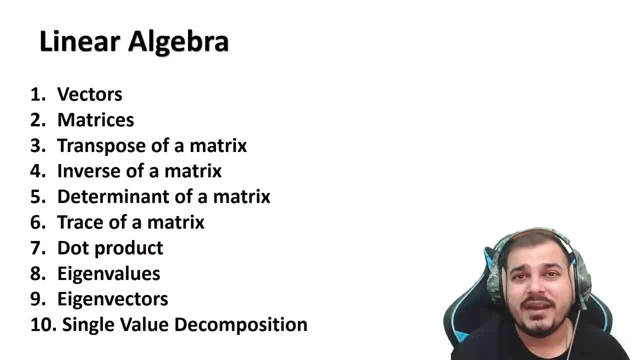 One is vectors: matrices transpose of a matrix, inverse of a matrix, determinant of a matrix, trace of a matrix, dot, product eigenvalues, eigenvectors, PCA, If you remember principal component analysis, which is a very amazing dimension: tree reduction. 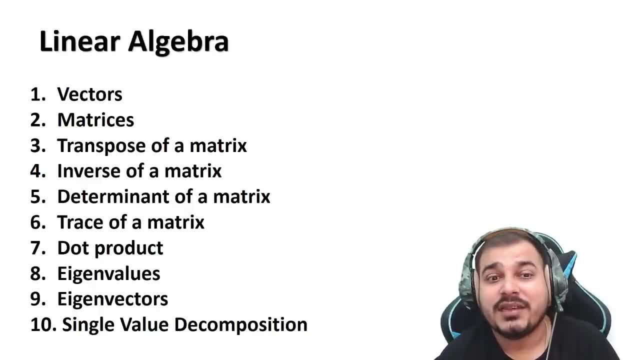 algorithm in machine learning. their eigenvalues and eigenvectors will definitely be used. Single-value decomposition: this is a pretty much important right If you really want to do the dimension tree reduction, And I'm not saying that this is only the thing, but these are the main things that you'll be using for most of the time, right. 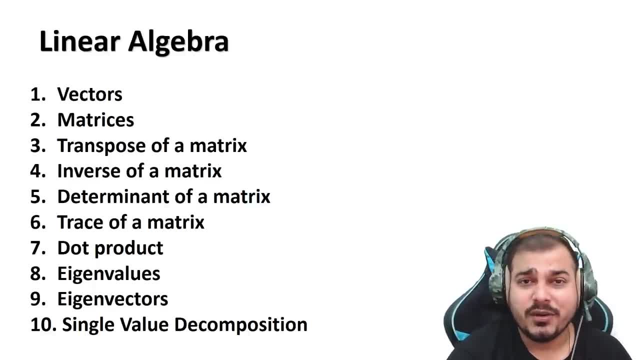 And most of the interview questions will be related to something like this. They'll try to understand what is vectors, what is scalar, how does eigenvalue, eigenvectors actually work? Everything they'll try to ask with respect to that. This is the basic thing, And when you are learning deep learning, probably you're learning some of the machine learning algorithms. 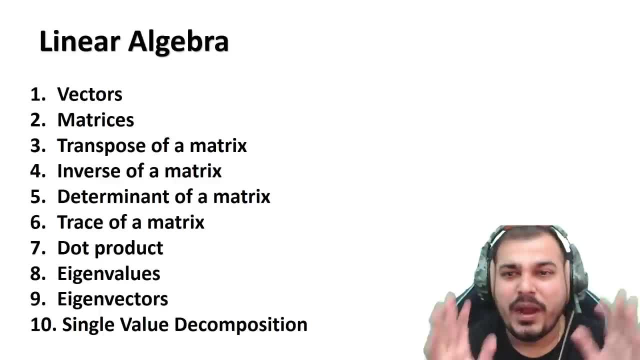 So you know this is the basic thing that you can learn on the algebras, And so that's a general theory, And you can learn this particular topic separately, How. I'll tell you where, or you can actually refer to everything I'll try to tell you. 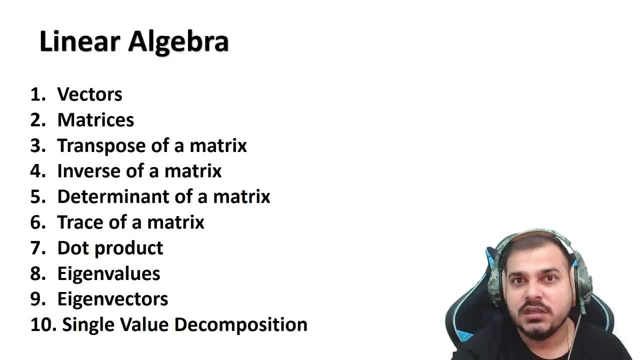 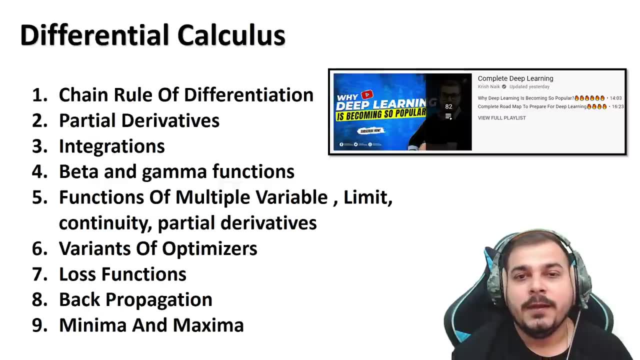 But understand. this is the smartest way to learn quickly anything. So first is linear algebra. Definitely, these are some of the topics that I have written and remember. I'll also try to convert this PPT into PDF so that I'll give you this link. You can actually see to it, Okay. 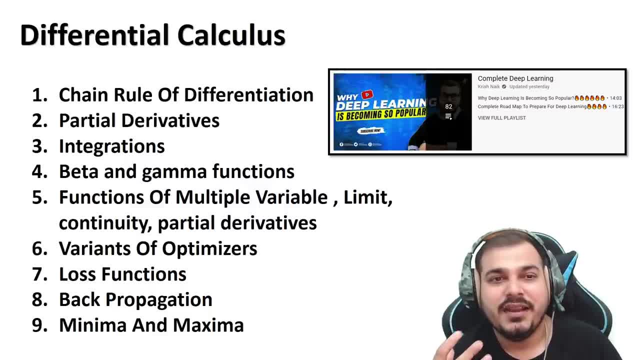 Now coming to the next one: partial derivatives- integration: right, Beta and gamma function. functions of multiple variable limit to continuity. partial derivatives- variants of optimizers. There are so many optimizers that are used, And these are some of the applications. 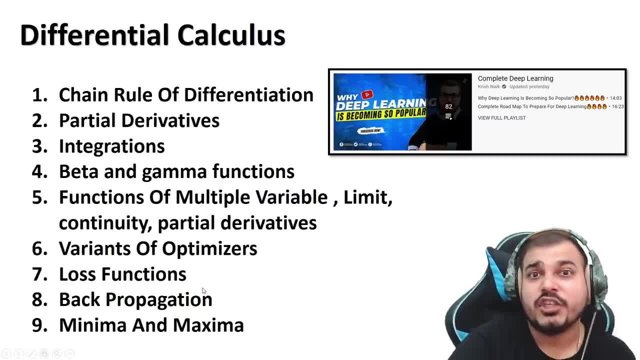 When I say variants of optimizers, loss function, back propagation, maxima and minima. these are some of the applications for this particular calculus that we basically use in deep learning. If you go and check out my complete deep learning playlist in my YouTube channel, guys, 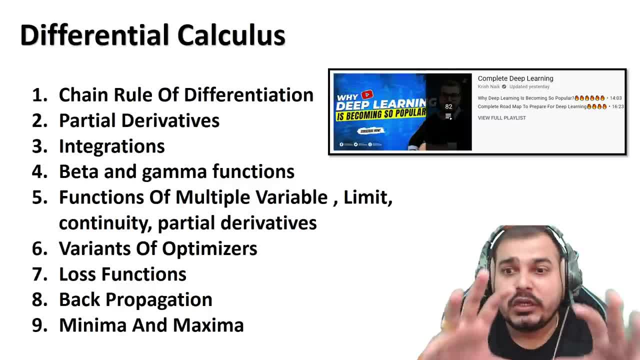 what I have done is that I have combined everything. Suppose if I'm teaching you that, how does a neural network work? I've actually combined all the calculus part inside this, Like there is a concept which is called as weight updation formula, And I've actually shown that. 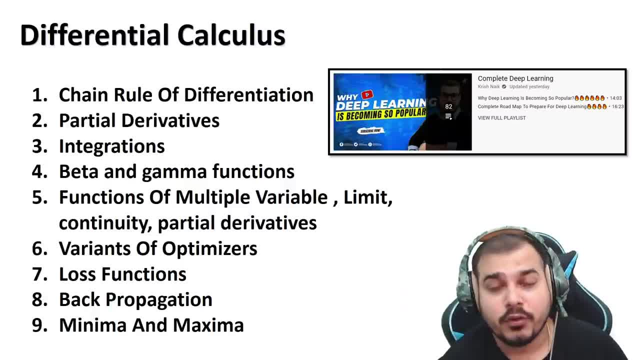 how does partial derivative or chain rule of differentiation actually happen over there while they are actually calculating the slope? So I have definitely made this as a story And that is the way that I've actually taught, So people should also think that learning should happen in that particular manner. 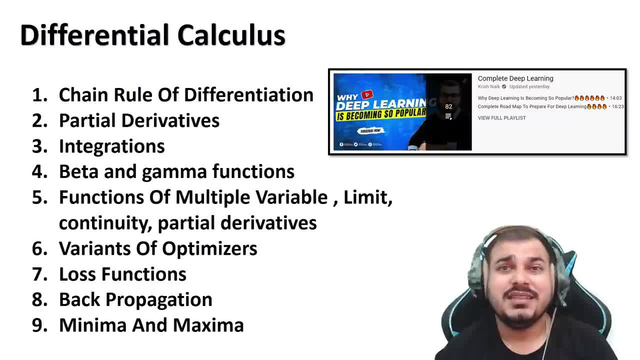 Otherwise it will definitely take one year if you are trying to learn all these things separately and then seeing that how it is basically applied in data science. Right, So you just go and watch my deep learning playlist. guys. If the first topic in deep learning playlist 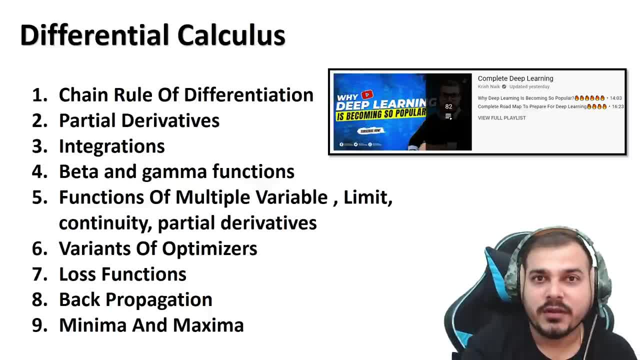 probably is that: how does a neural network work? So there, I've included some of the maths. Then, how does back propagation actually happen? I've included some of the maths over there. Okay, Calculus, definitely Right. And then, if you go to the next topic, 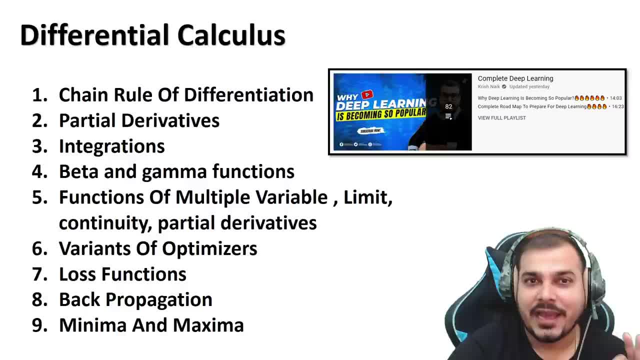 I should have written over here differential calculus, but instead I could have written calculus, So I'll just make these changes Right. When I started teaching you different types of optimizers, there are different types of optimizers: Gradient, descent, AdaGrad Adam. 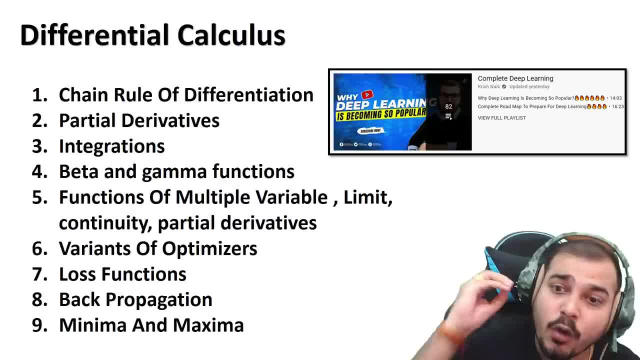 Different optimizers are there, And there you'll be able to understand how calculus is amazingly used. There's an application which is called Minima and Maxima, which is final goal of training the deep learning models. So what I've done, I'm not teaching you separately. how does this happen? 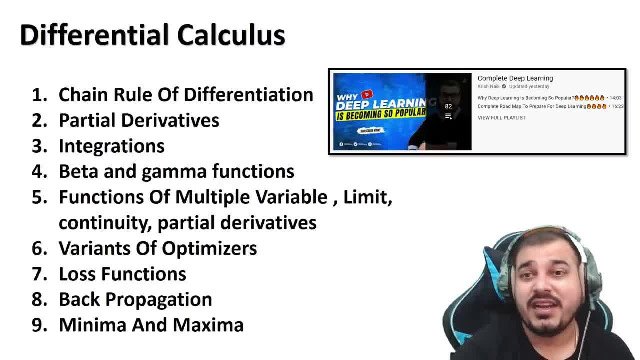 Instead, I'm teaching you along with the subject, So you should definitely have a look onto that, And that is how the learning will quickly happen. Right Now, let's go to the third part. I think most of the important things I've actually covered over here. 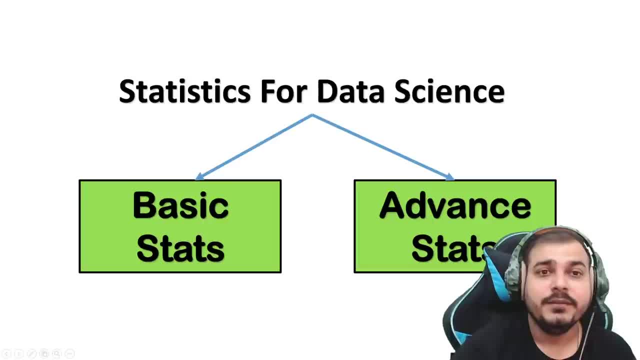 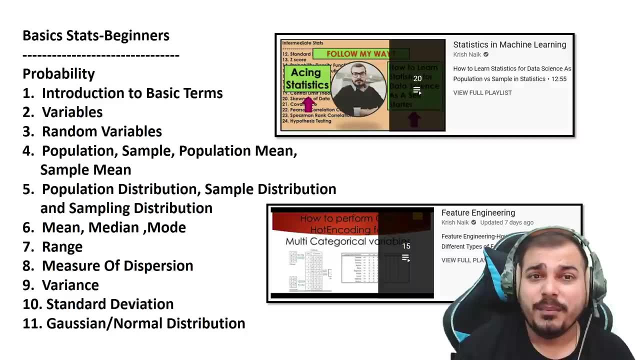 which is very much applicable to data science. Now, if I go to the next step, stats and statistics, I'd like to divide this into two parts. One is basic stats and one is the advanced stat. In basic stats there are terms like probability. 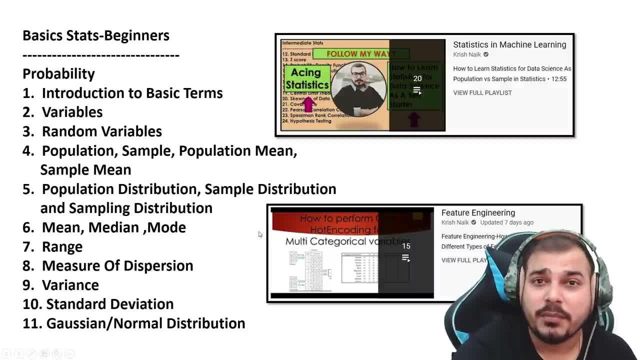 introduction to basic term: variable, random variables. what is population sample, population mean population distribution, sample distribution, mean median mode, measure of dispersion, variance, standard deviation, Gaussian normal. all these things you'll be able to find out in these two playlists. 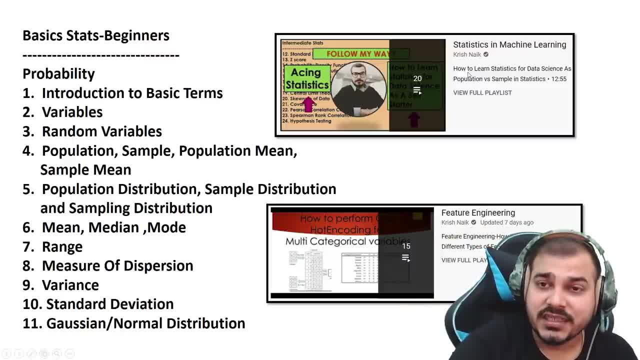 That is, statistics in machine learning, feature engineering. Now, in statistics in machine learning, what we have actually done is that I've explained you the theoretical part And in feature engineering you'll be able to see that how we are able to apply this in practical purpose. 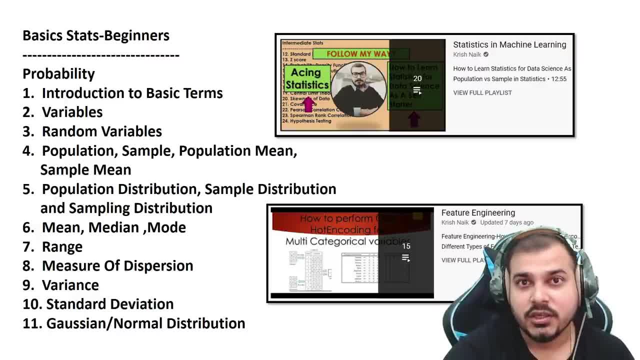 Even there is a playlist on EDA, exploratory data analysis. So this is specifically used most extensively used to do the EDA part, to do some of the feature engineering part. So definitely this is the basic stats that is being used. 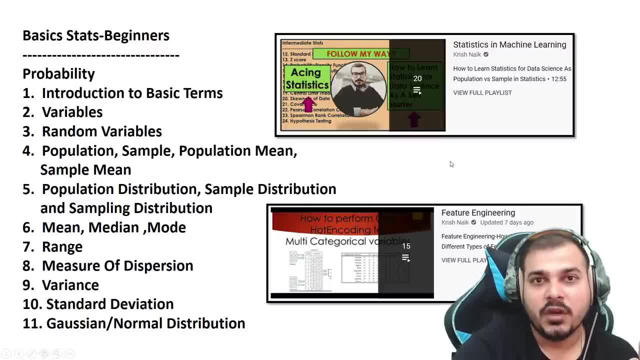 So this is the basic stats that is being used. So this is basically required for you all to know. You know again, if you are going to prepare for data science guys, one suggestion that I really want to give you guys: don't make it as an extended way. 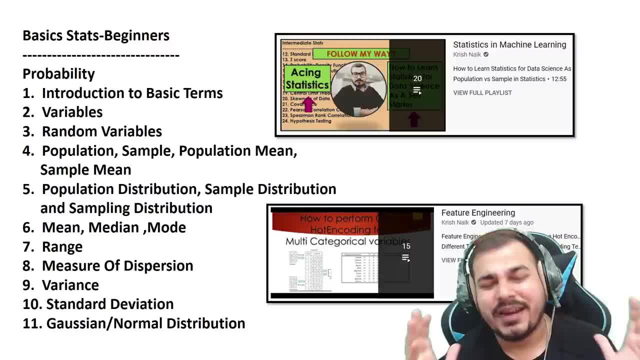 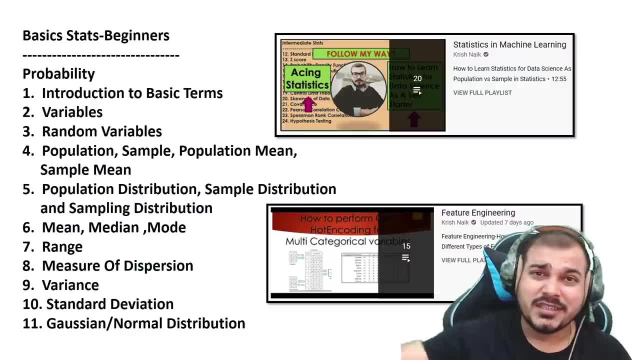 Try to be smart, try to complete the portion. try to do that much so that you'll be at least able to get the job and you'll be able to work quickly. Right, I know end-to-end projects is actually required, but before that you really need to complete all this machine learning projects. 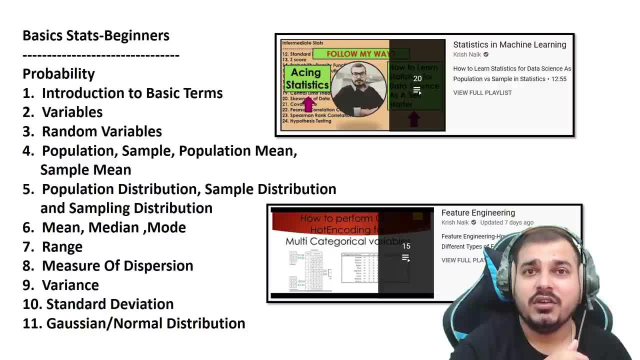 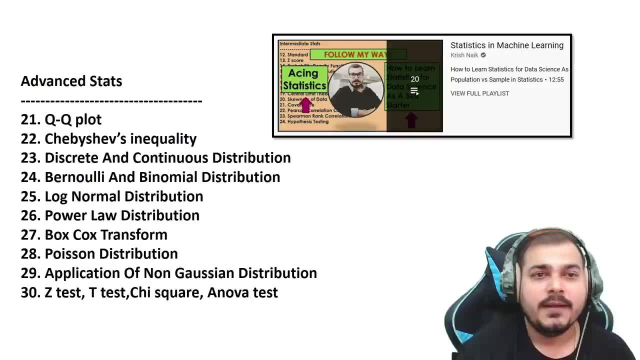 and all sorry machine learning algorithms, stats. you know you need to complete how you are going to apply linear algebra and all, And if you are able to learn in that specific manner, it is very, very good right. 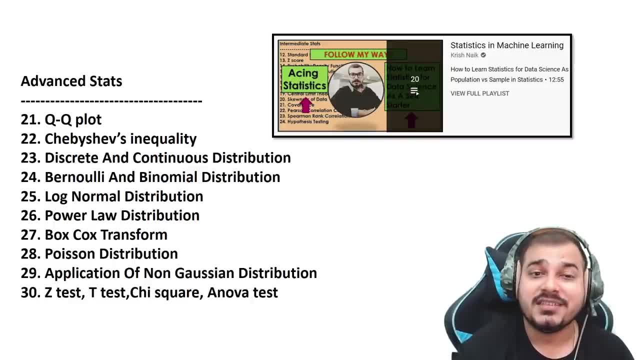 Now coming to the advanced stats. So here you have QQ plot. chevy names: inequality, discrete and continuous distribution, Bernoulli and binomial distribution log. normal power law. Cox box. Cox poison distribution application. non Gaussian distribution Z test. 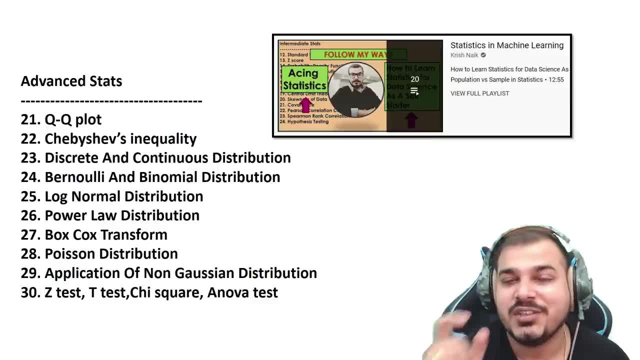 T test, chi-square test and over test. this Z test, T test, chi-square and over test is a part of inferential statistics, where you take a population, you take a sample and you make some conclusion for that particular sample by performing some experiments like this. 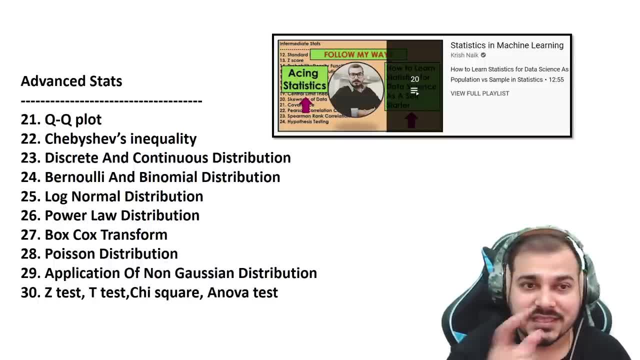 This kind of Z test, T test, chi-square test and all right, And this is also definitely being useful in EDA part When I say about QQ, plot chevy names, inequality, log, normal distribution, your data is having different, different distributions and all. 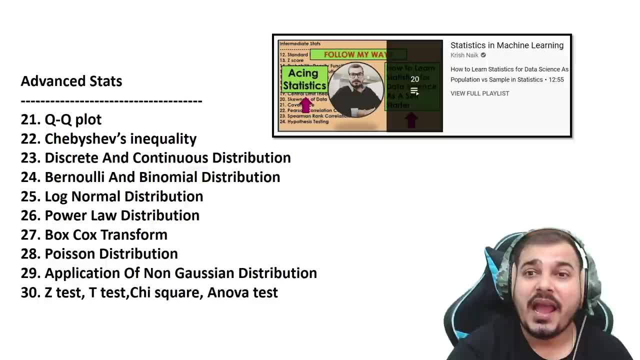 And again, all these things is covered in my statistics in machine learning and EDA playlist. Okay, So the reason why I'm making this entire video is that, guys, to make sure that you're learning, should be pretty much efficient. Now let me talk about the sources. 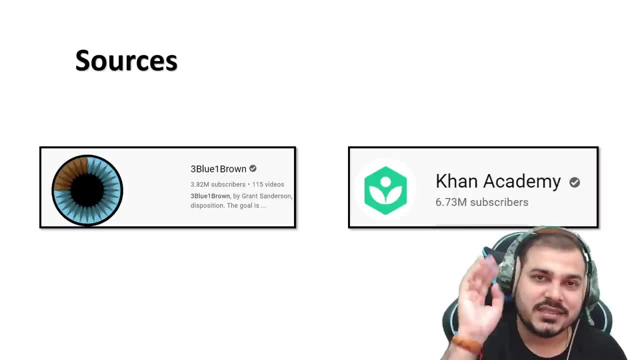 I've already told about my playlist, but this two sources, that is, three block, three blue, one brown and Khan Academy will definitely help you to understand all these things. That is, linear algebra, calculus, even stats. Okay, Now when to refer. 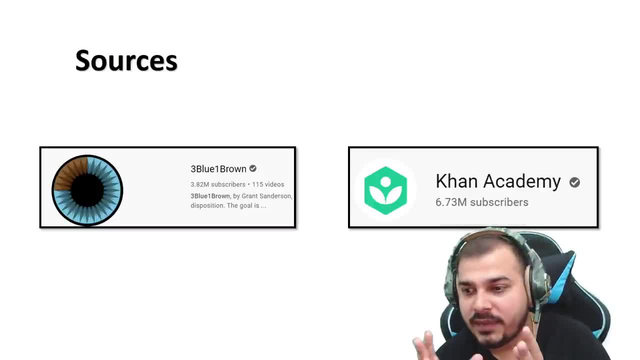 how to refer. I'll tell you. suppose. just imagine that you're seeing my linear regression. Suppose you are seeing my one of my video in PC or a principal component analysis. So in principle, component analysis. suppose I have discussed about eigenvectors and eigenvalues. 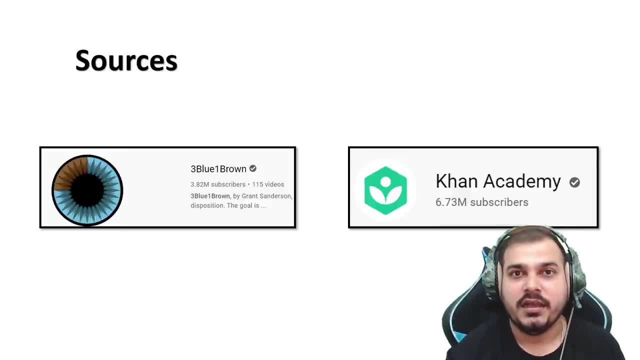 Then I'll not say you what exactly is eigenvectors and eigenvalues, values, right? I'll not be able to tell you. if I'm actually explaining you something, I'll tell you that here we use some kind of vectors, here We use some kind of scalar, and this is what the formula is. 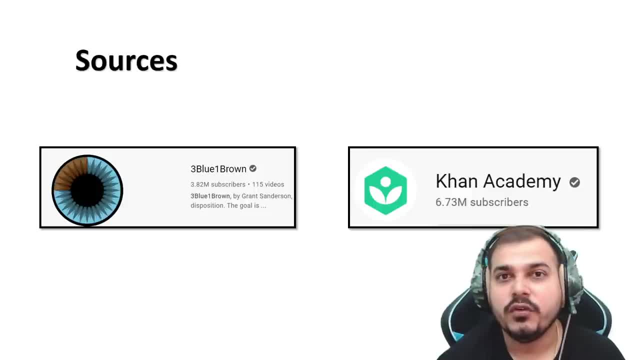 I'll definitely not be able to derive the formula over there. So what do you need to do? Is that okay? You have not understand that. How does that eigenvectors comes, or how does how does better behave? How is this formula derived? 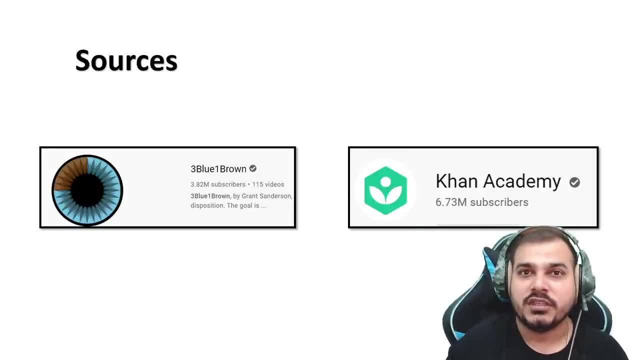 You can definitely watch the Khan Academy or three blue, brown, one brown series, because they have explained in an amazing manner till the crux. Okay, I'm not telling you to just go see in Khan Academy. Everything is there with respect to linear algebra. 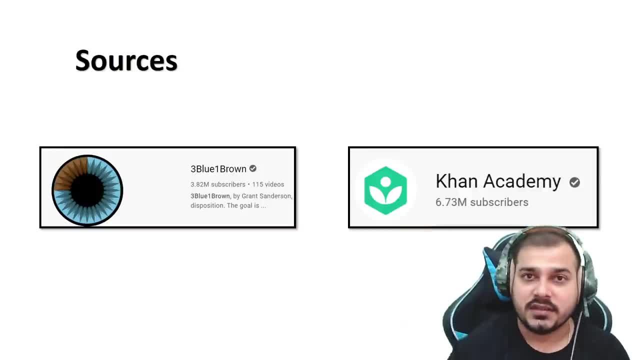 statistics, everything is there, but you need to spend time to learn all these things. But instead I'm telling you to go and learn in that way that suppose, if you're learning a topic, suppose I'm learning a topic with respect to PCM. 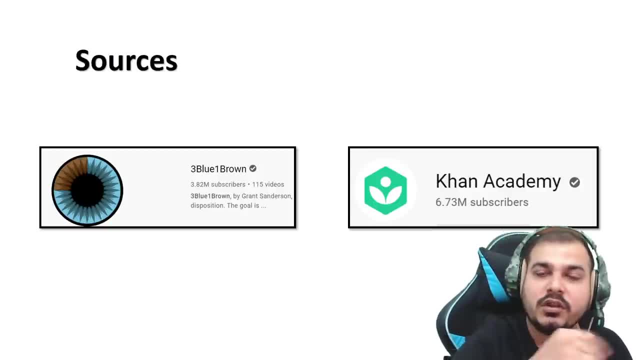 Okay, And if there is something like eigenvalues and eigenvectors, I'll go into the Khan Academy and there is a topic on that also in the YouTube channel. I'll go and read it, I'll try to try to understand more in depth and then I'm pretty much sufficient. 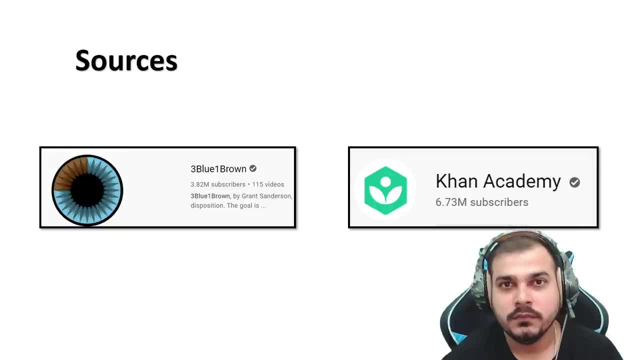 because I will be able to understand that particular algorithm In an amazing way. right, Suppose I want to understand partial derivatives. Suppose in back propagation we do partial derivative and partial derivative, We calculate the slope and then we try to reduce the weights. 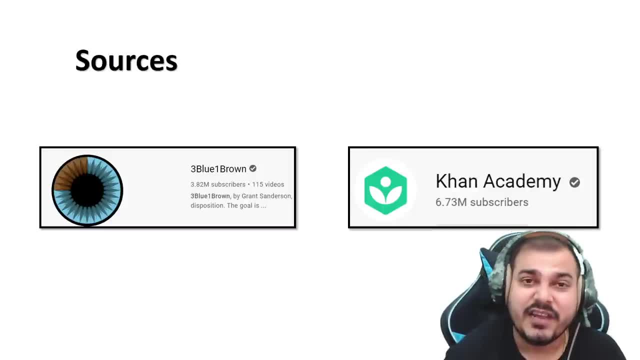 Okay, This is what happens in deep learning. Now, how does this partial derivative happen from scratch? If you want to go and check it out, check three blue, one brown series or Khan Academy. They're definitely one topic will be there with respect to that. 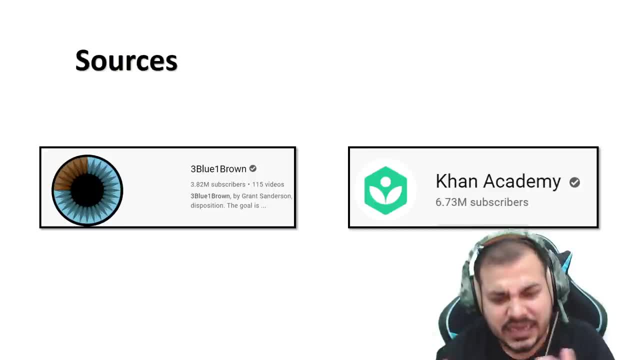 Also in stats. Also, suppose you want to understand one topic in completely in depth and probably you're following my playlist. You're learning over there and suppose if you have facing some problems, go over there and try to learn it from there, only to make your base stronger where you are actually. 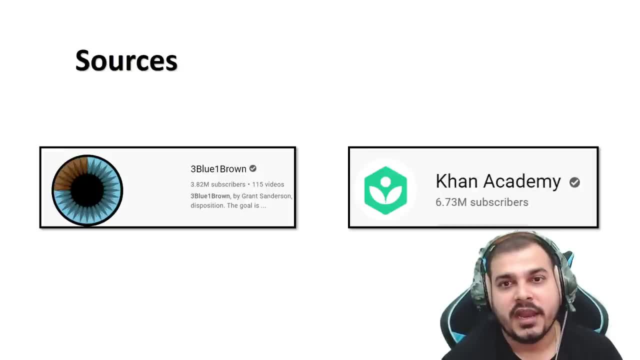 confused. You have to definitely follow this particular pattern right. This to YouTube: Shannon is pretty much amazing. One is Khan Academy and one is three blue, one brown. with respect to any kind of maths more depth, You really need to see some visualization diagrams and all definitely right, and I'd also like to prefer stats. 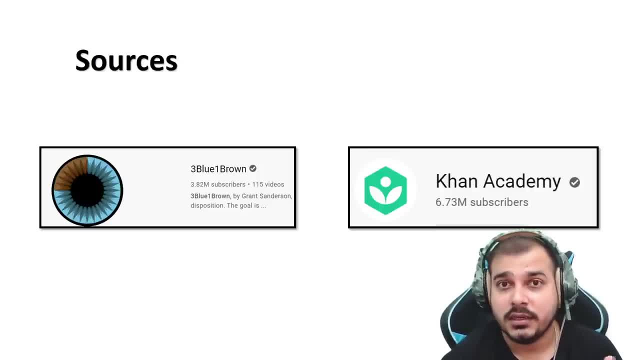 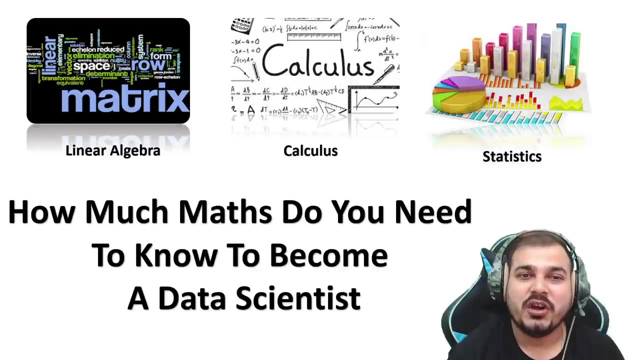 quests. You know, start quest is also an amazing YouTube channel Where a lot of maths, a lot of easy maths, will be actually displayed with respect to statistics, right? So this is what I would suggest you all to follow. This will definitely be helpful and this is how you can definitely make sure that this is what the math is. 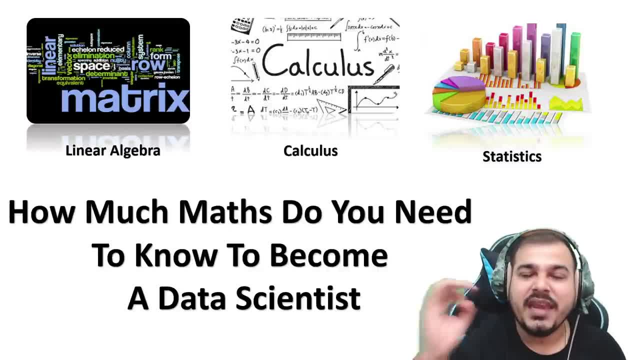 Basically. quite again, math is quite huge, but again, my main aim of this particular video is that try to learn data science in a quicker and a smarter way, so that you don't have suppose. just imagine you don't have much time, So 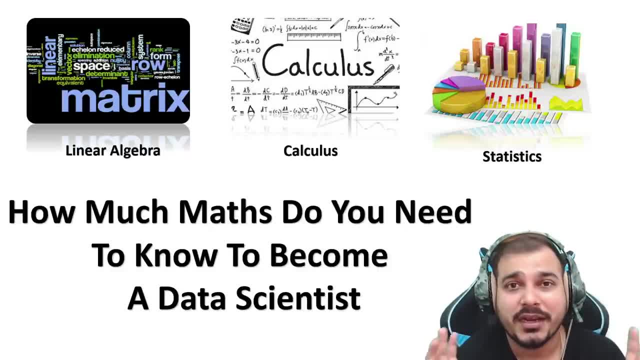 yeah, you have to be very much smart while you're learning things and you really need to complete it quickly, right, And that is the reason your school maths will also be coming in. You really need to have that particular knowledge also, but if you try to follow this particular pattern,